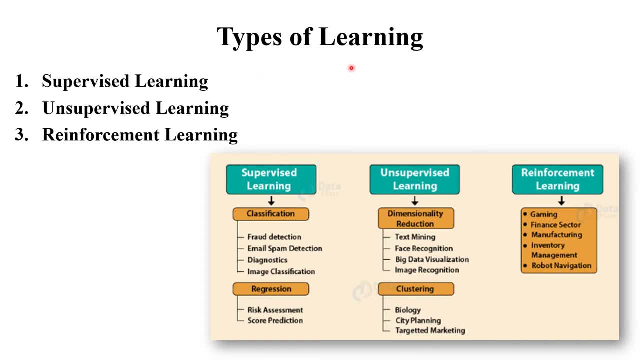 Okay, So the first type is type Types of learning. The first point is types of learning. So in machine learning there are basically three types of learning: That is, supervised learning, unsupervised learning and reinforcement learning. In this session we will learn about the first type, that is supervised learning. 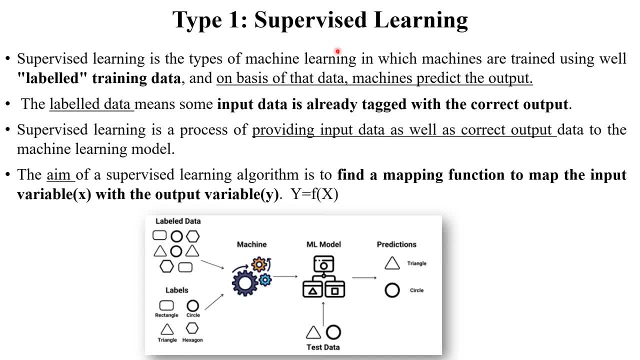 So what is mean by supervised learning? See, supervised learning is a first type of machine learning which machine are trained by using some label data Means we will pass as a information Input to the particular machine and the input is in the format of label data, For example, see in this diagram. here, Suppose there are two types. There is the types of input. Okay, Which input include label data and their image. For example, see here: this is circle and the label is circle. This is the image of rectangle and the label is rectangle. This we will pass the input to the machine. that is label data. 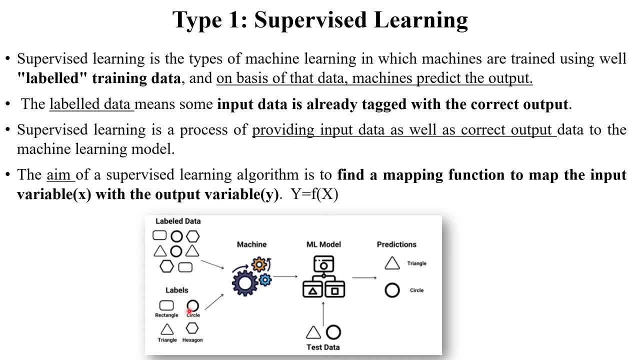 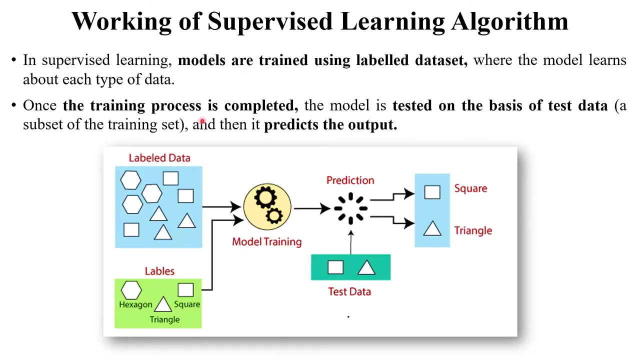 Means. we will provide the input data, as well as correct their output data to the machine. So this is a concept of supervised learning algorithm. we will pass label input data to the machine for training purpose. now, see here, this is just a working of supervised learning algorithm. so in 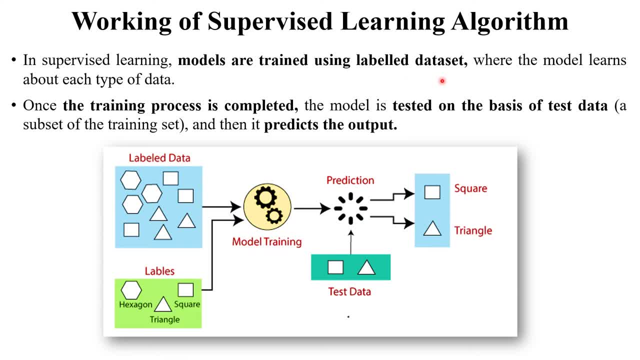 supervised learning models are trained by using label data. so where the models learn about each type of data- see here- this is called as label data and these are the labels and this combinedly is called as input. so in label data there will be a image of hexagon and their label is hexagon. the image is square, the. 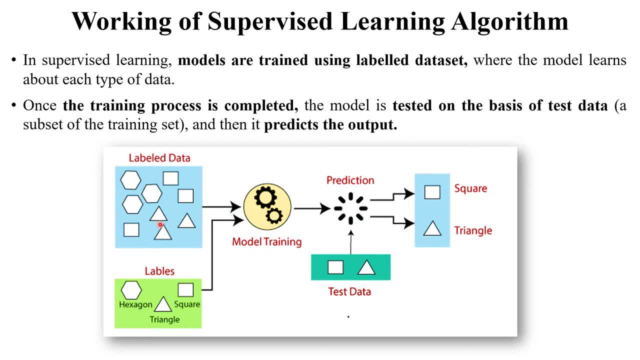 label is square. okay, and there is again another image is triangle and their image label is triangle. so we will pass this label data to the machine for the training purpose, so machine learn their features, their structure and the characteristics of each and every image. okay, and after that, by using testing, 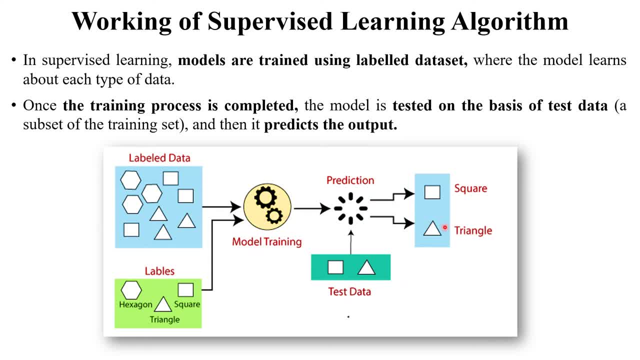 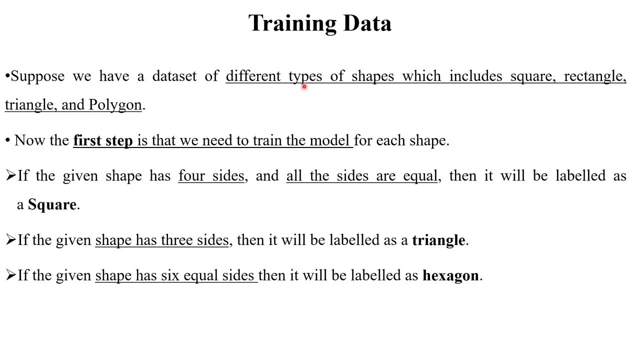 data set. we will test the particular images with the particular machine. that particular machine can be trained by properly or not. okay, so this is a working of supervised learning algorithm. now the first step is you need to train the data. okay, there is a label input data set you. 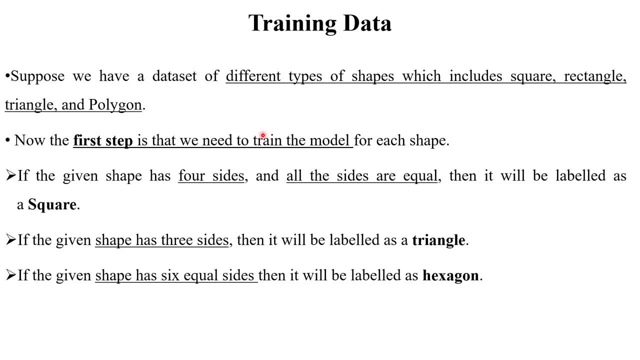 should pass those data set as an input to the machine, right? so first thing is you need to train the machine. suppose we have a data set that is different types of shapes, right? that is, square, rectangle, triangle and polygon. so in training data set machine can be trained by using their features. 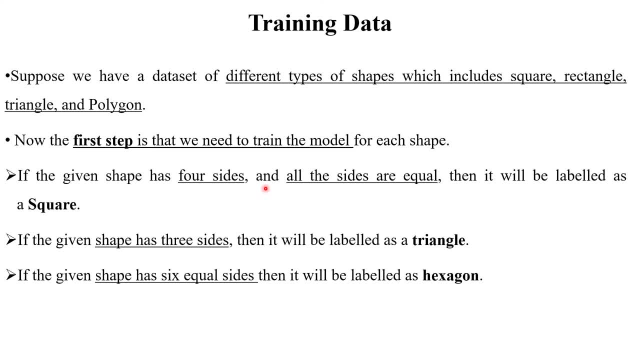 for example, if the given shape has four side and all the sides are equal, then it will be labeled as a square. again, if the given shape has three side, then it will be labeled as a triangle. and if the given shape has six equal sides, then it will be labeled as a hexagon. so this is called a training means. machine can be. 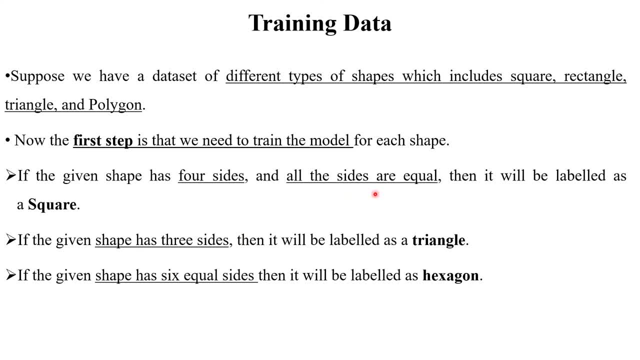 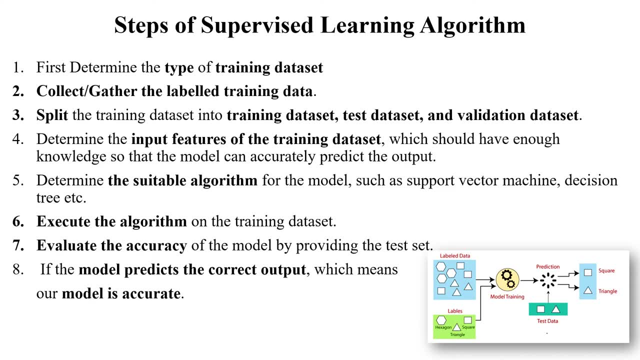 trained by using features of those particular images. okay, and the features is mapped with the particular labels. this is called as training data set. so first, these are the steps of supervised learning algorithm. see here. first, you need to determine the types of data set. okay, whether your data set regarding to 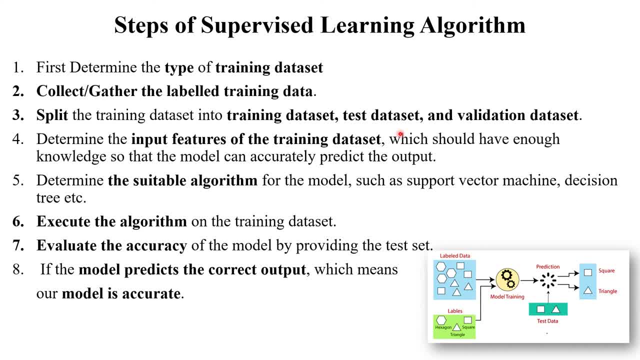 the students regarding the shapes of the particular images, then fruits images, etc. so you need to identify what is your particular training data set. then you need to collect and gather a label training data set and then you need to determine the types of training data set. okay, because in supervised learning, 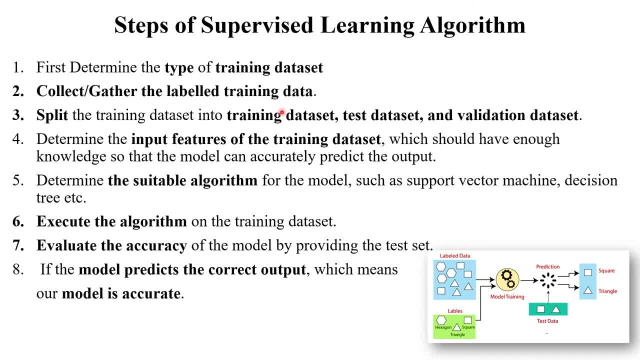 algorithm. we will use labeled training data only. now your complete data set can be divided into the three parts, that is, training data, testing data set and validation data set. okay, so we will use, suppose, 75% images for training purpose and, for suppose, 25% images for testing purpose. okay, now the fourth step is. 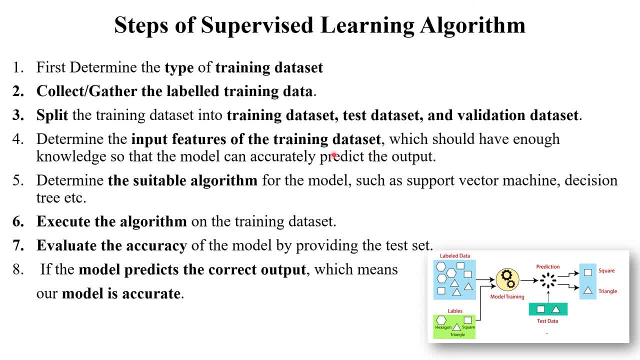 determine the input features of training data set. okay, miss, machine can be trained by using some suitable algorithms, like we will use support vector machine decision tree, this kind of algorithm, for training purpose. so machine can be trained by using the features of those images right. after that you need to execute the algorithm for the training data set right, and 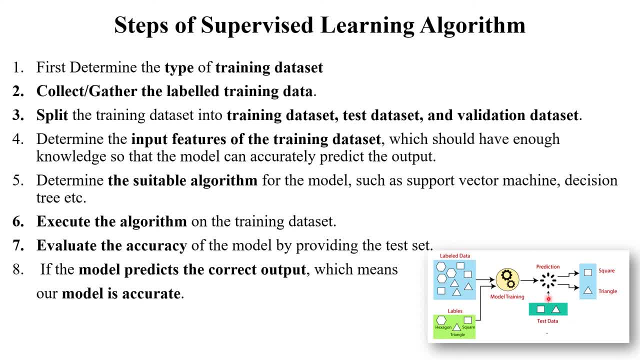 after training is completed you need to test different images with the machine. suppose you should give the particular square image to the machine. then the particular model predict the results, that this image is called a square. suppose when you pass the circle image to the machine, but your model is not trained with the circle image, right? so 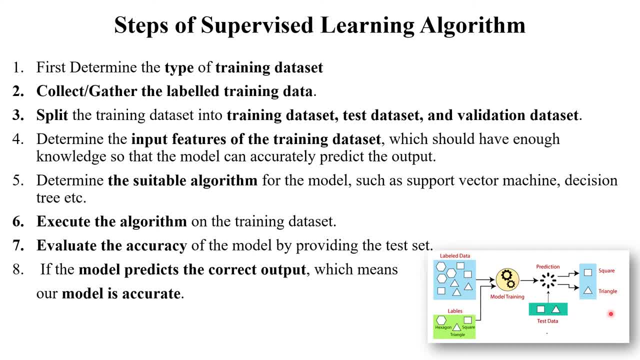 it shows you that the particular area will be generate right now. suppose you should pass the triangle image to the machine now? model predicted that the particular image is called a strangle, so this is called as supervised learning algorithm. if the particular model generated the accurate result, so that can be decided by the accuracy of the model how the 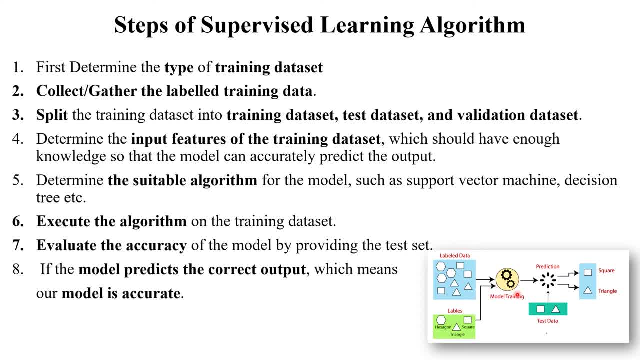 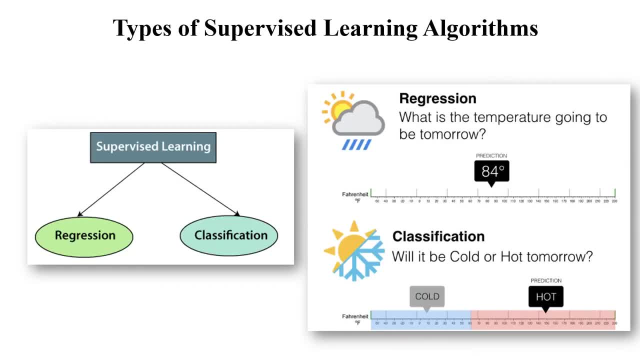 particular model predict the correct output, which means the model is accurate, clear. so these are the steps of supervised learning algorithm. now there are two types of supervised algorithm. one is regression and another is classification. so here there is just a simple difference between regression and classification. so classification means unit. 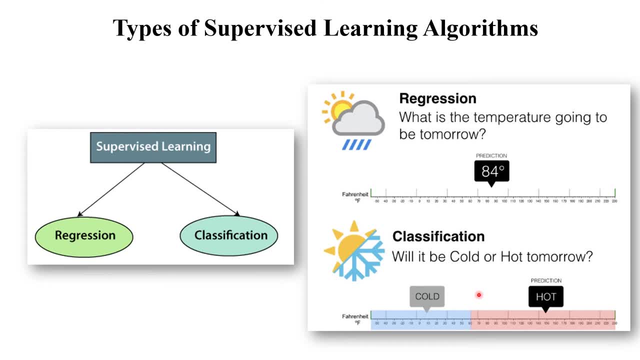 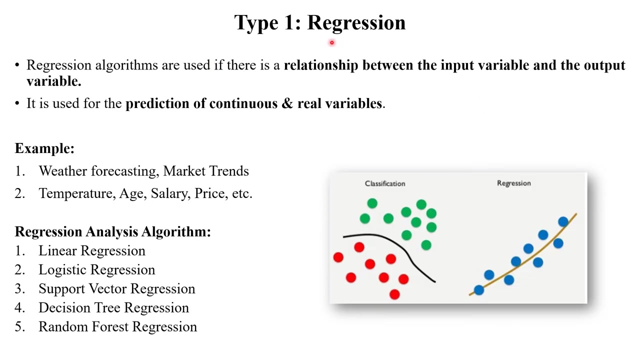 classify the data. either a temperature is cold or hot, right, so this is called as classification. but regression means the value is continuously change, for example temperature. so temperature is continuously change as per the morning, afternoon or evening, right, so this is called as regression. so let's see in detail. so the first type of supervised learning algorithm is regression. 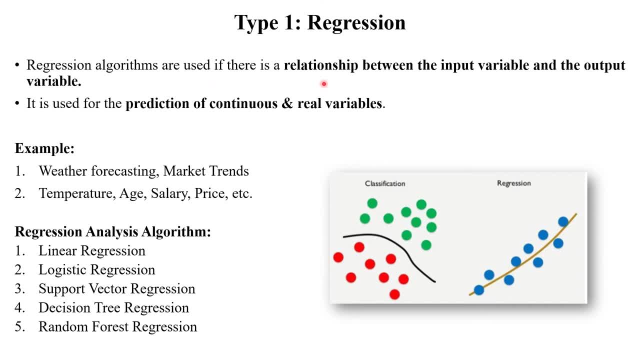 now, what is mean by regression? so regression algorithm is used if there is a relationship between input variable and output variable, okay. and it is used for the prediction of continuous and real variable, for example, weather forecasting, temperature, right. temperature is continuously change. now next one is age. okay, your birth date and age. both variables are depend on each other. 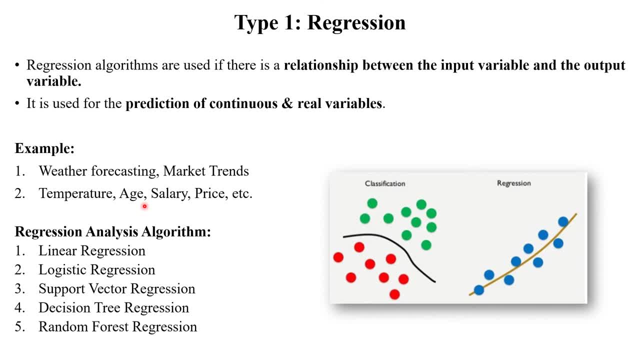 means according to your birth date, you should calculate the age, right? so these things are depend on each other and this- the age- is continuously change, right? so this is called as regression. then there is a market trends means stock price, share price. this is also a changing values and that will be depend on the market. then salary price, right so? 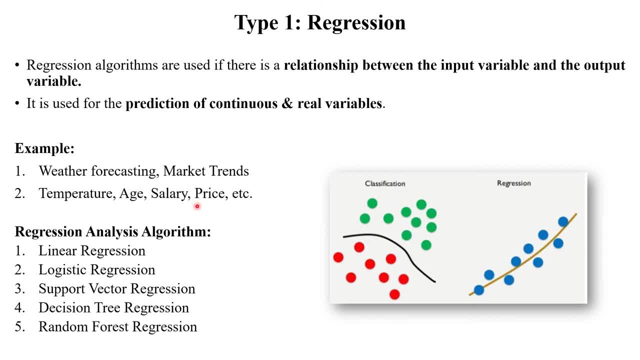 this is a concept of regression and for calculating the regression we will use different analysis algorithm like linear regression, logistic regression, support vector decision tree and random forest regression. so we will learn all those algorithms in your third unit. your third unit is called as regression. okay, next, now the next type of supervised learning. 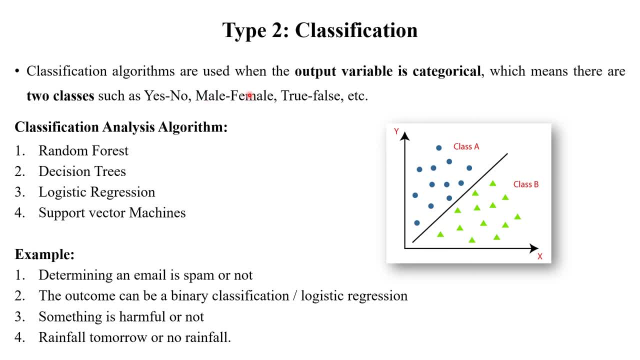 algorithm is classification. so classification of algorithm is used when output of variable is categorical, which means there are only two classes, such as yes, no, male, female, true, false, etc. so this concept is called as classification and there are different classification analysis algorithm like random forest, decision tree, logistic regression and support vector machine. so we will learn this algorithm in your second unit. 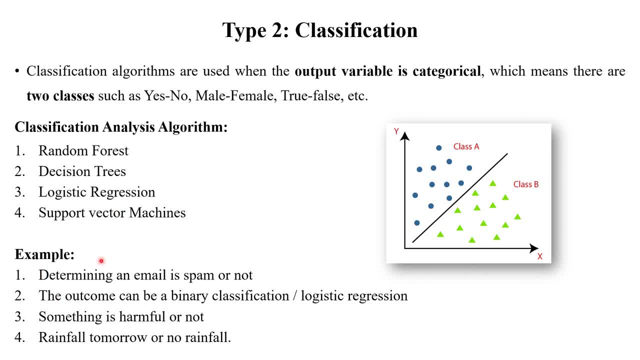 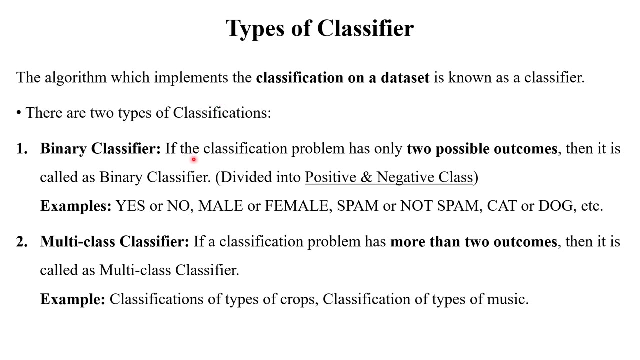 your second unit is classification. okay, now see, these are the some examples of classification, like determining the email is spam or not, then outcome can be binary classification or logistic regression. then something is half full or not, rainfall tomorrow or no rainfall, right? so these are the examples of classification. now, in classification there are two types of 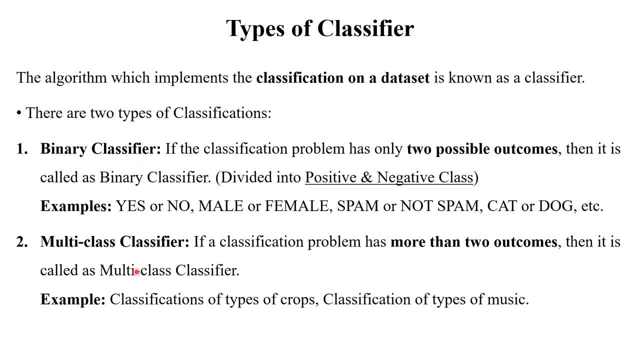 classifiers are used. one is binary classifier and another one is multi-class classifier. okay, so this algorithm which implements the classification on the particular data set: okay, and that's why they use a classifier. so binary classifier means if the particular classification problem has only two possible outcomes. that is yes or no means there is only two. 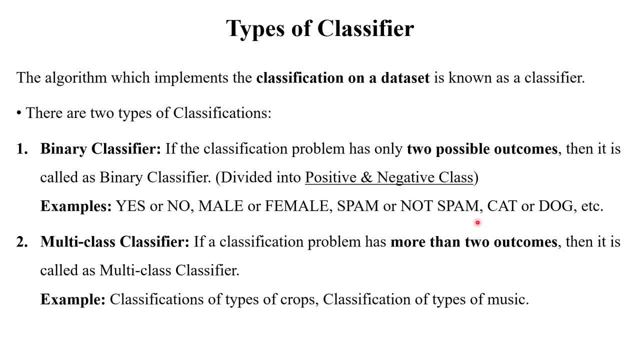 possible outcomes: male or female, spam or not. spam cat or a dog, right, so this is called at that time. this data can be represented by using binary classifier. okay, and multi-class classifier means if the classification problem has more than two outcomes, which is called as multi-class. 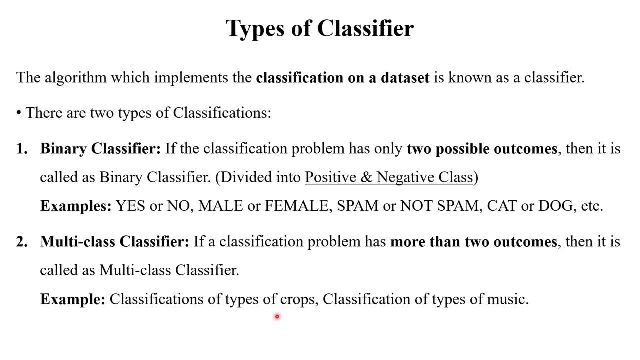 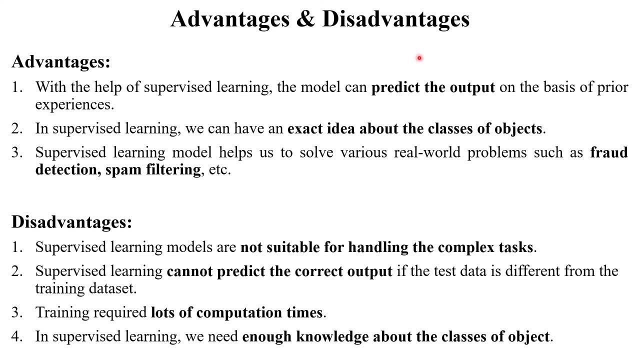 classifier. for example, types of music, types of crops mean there are multiple types, are there right? so that can be denoted by using multi-class classifier. okay, now the advantages and disadvantages of supervised learning algorithm. so, with the help of supervised learning algorithm, we will predict the particular output. okay, on the basis of your experience, means in supervised 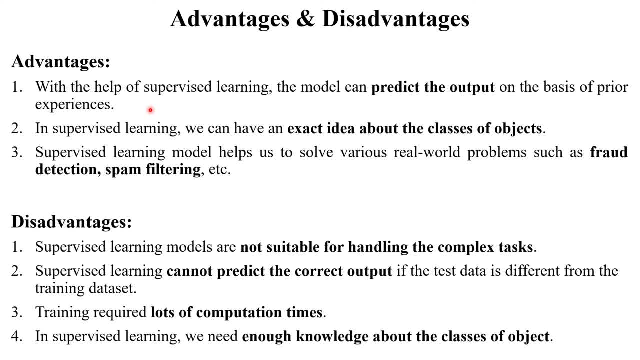 learning algorithm, we will pass labeled input data. that's why we will predict the correct output that will be matched with the particular label. so this is the advantage of supervised learning algorithm. now, uh, in supervised learning algorithm, we will solve supervised learning and revised learning algorithm. also, sometimes, very often, probability- like if we anywhere in coded fields above that is used to predict the rises, the particle data- these digits will match the output data, like this flag倉磊ž čibins praying ° eg. 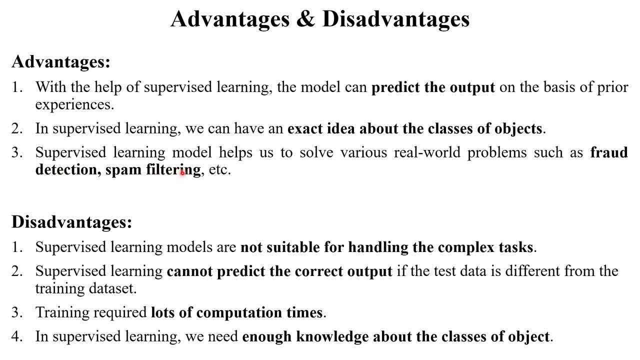 real-world problems like fraud detection, spam filtering, etc. now the disadvantages of supervised learning algorithms are: this model is not suitable for handling the complex task. if the particular data set labels are not given, okay, at the time supervised learning algorithm is not used. it required only label data and supervised algorithm cannot predict the correct output if the test data 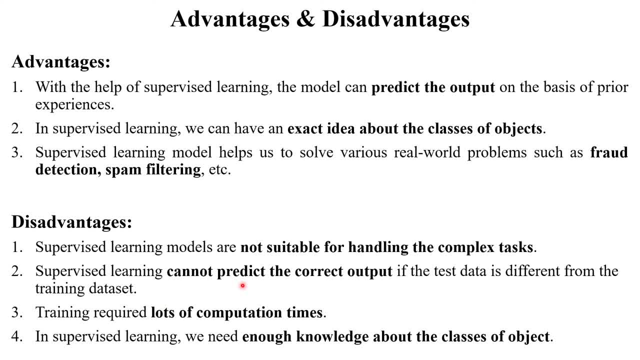 is different from the training data set means, suppose you should train the machine by using apple images, okay, and for testing purpose you should use mango images. so at that time it cannot generate the correct output. okay, it can't predict the correct output. so this is the disadvantages of 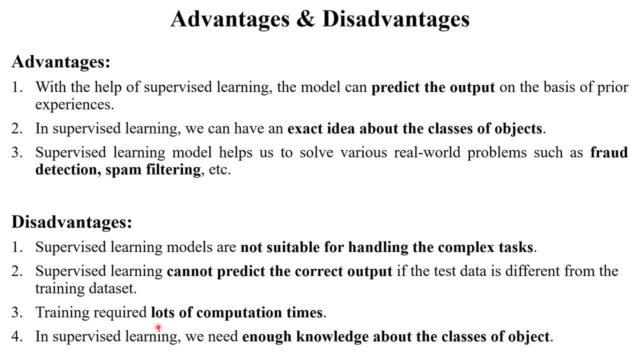 supervised learning algorithm and sometimes training required lots of computation time. for supervised learning algorithm it must to first follow training phase. okay, after that follow the testing phase. so sometimes it required a time. then we need to enough knowledge about class of objects. means for supervised learning algorithm we need to require. 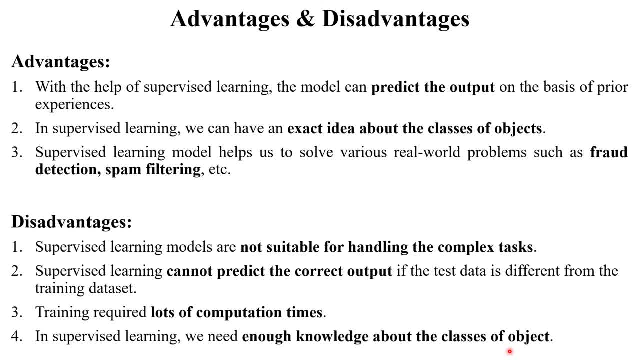 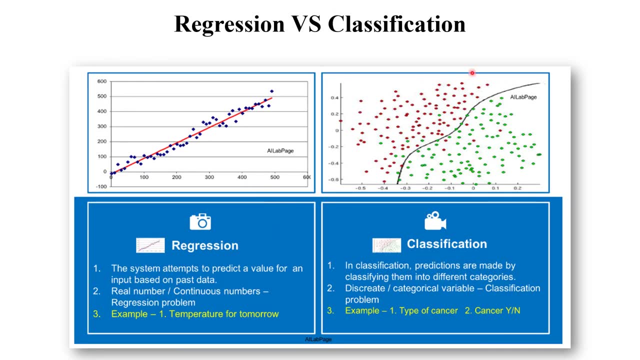 the particular classes of objects means, for example, the particular image of fruits and their labels. okay, we have the approximate knowledge of each and every прид, autonomous. so these are the disadvantages of supervised learning algorithm. now see here, This is just the difference between regression versus classification.